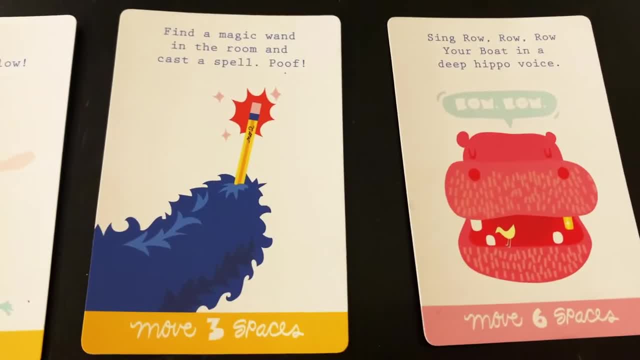 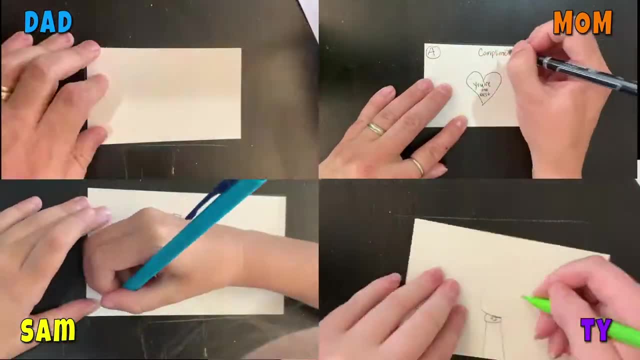 Ty wasn't bored with it, So we played it a lot, and it doesn't have an expansion pack, So we decided to make our own version. Yeah, What's it called, Sam? Ours is called Tortoise Town- Tortoise Town. 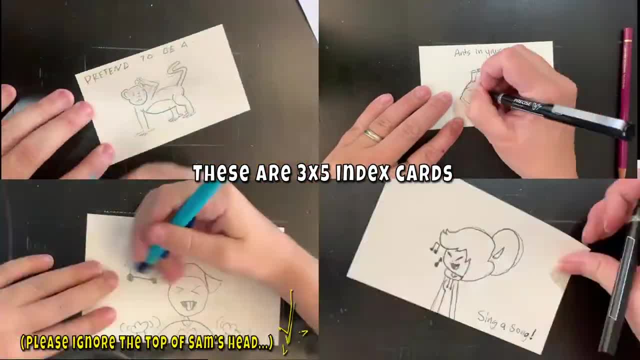 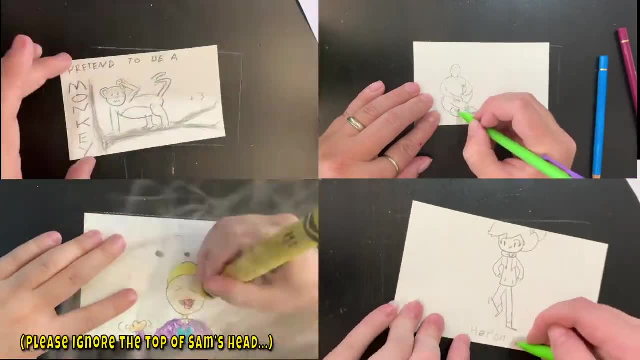 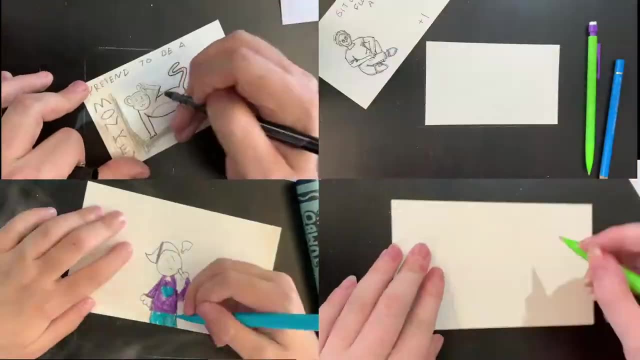 So we're drawing our cards. We all got to come up with ideas for cards and how to illustrate them and completely customize our own game experience. The way that Silly Street works, and so, therefore, Tortoise Town works, is each card has you do. 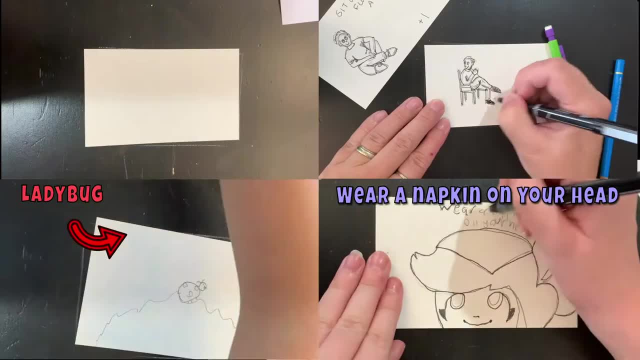 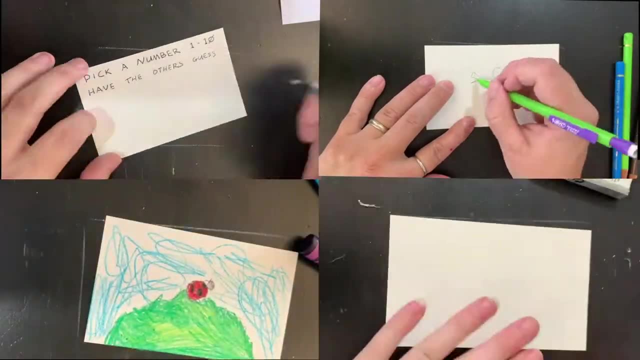 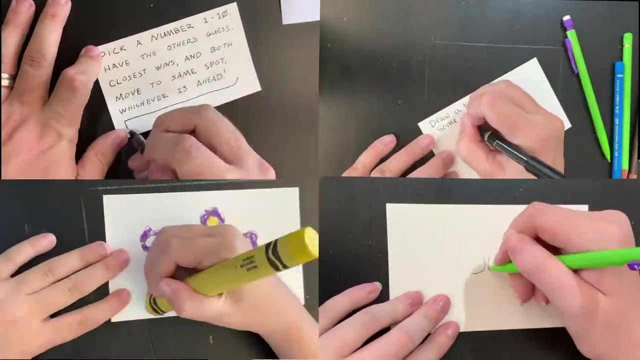 something and, based on what it is, you get a certain number of spaces on the game board. Tyler's doing black and white kind of pen and ink, illustrated style, And Sam's are crayon style. I've got more of a colored pencil and ink or just ink. Yep, that's what I was doing. 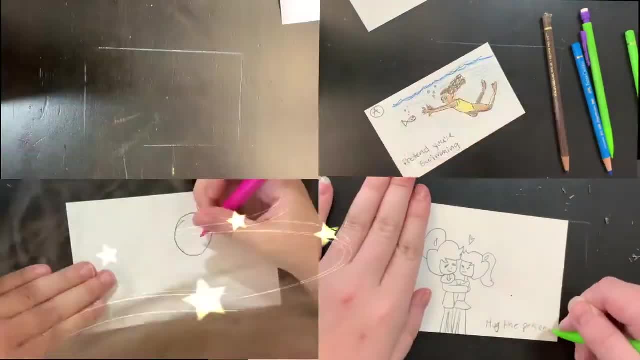 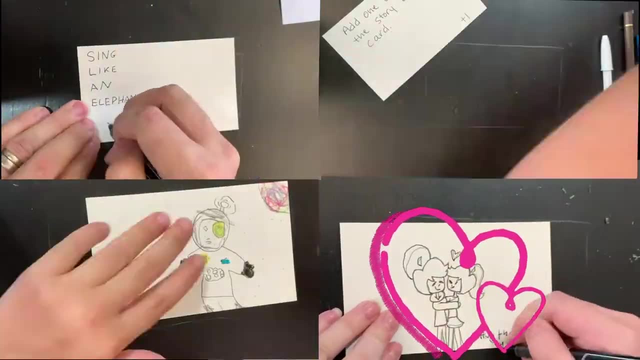 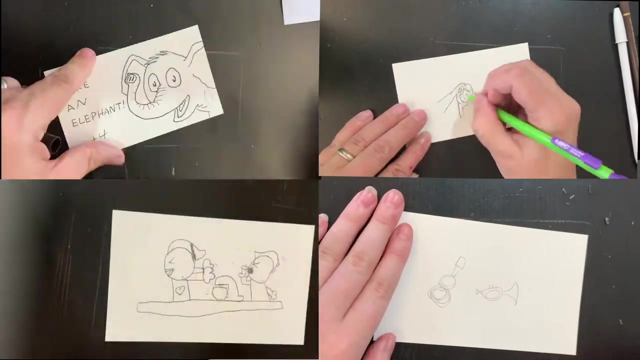 too, And we all came up with some ideas. and I came up with some ideas and shared them and they're all kind of fun, silly things that I knew would work for us And the point of the game is to be silly. So the sillier your card or the sillier you can make, whoever's playing your card? 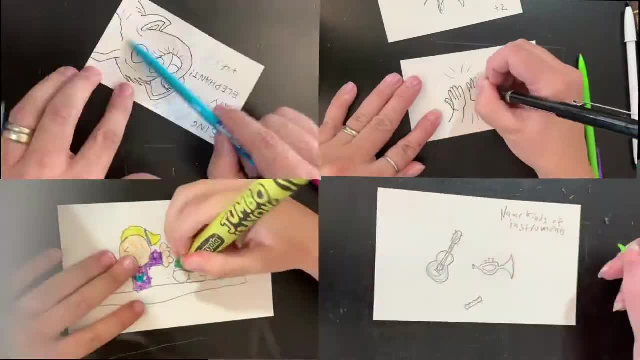 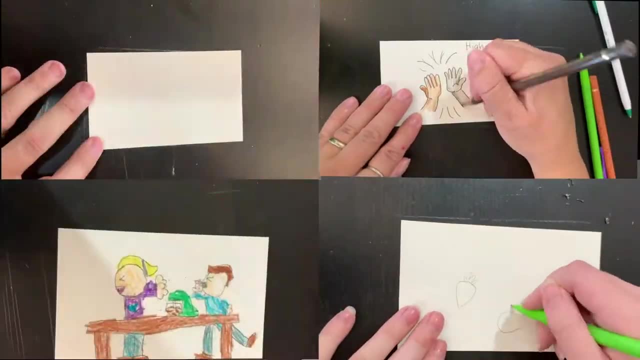 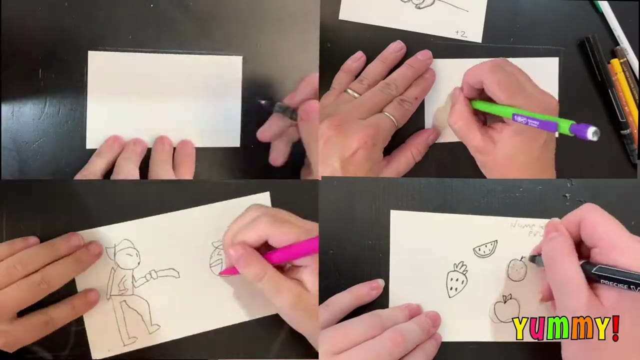 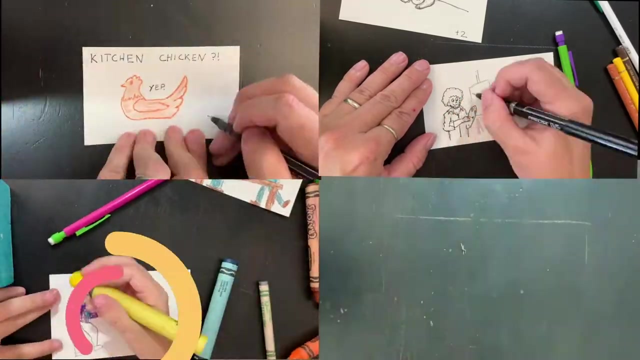 act, the better. For sure, I came up with the idea of a reverse card Like an Uno. Yeah, Yeah, When we played it, we actually got that one early on, So we had to switch. we switched directions before I even got a single turn. Yeah, But it's nice because now every time we play it we can 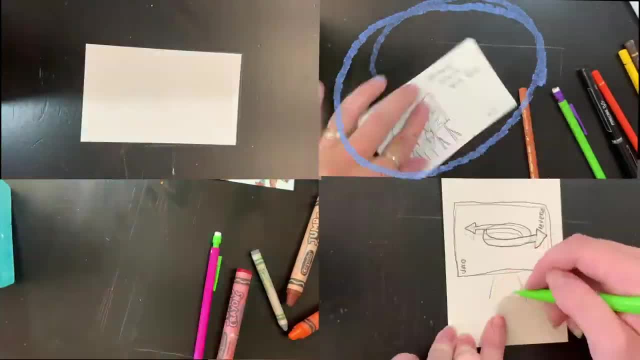 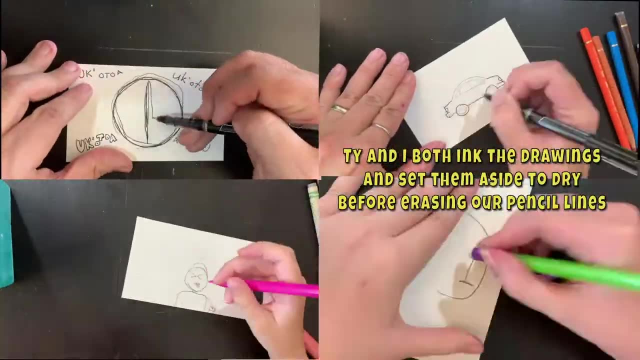 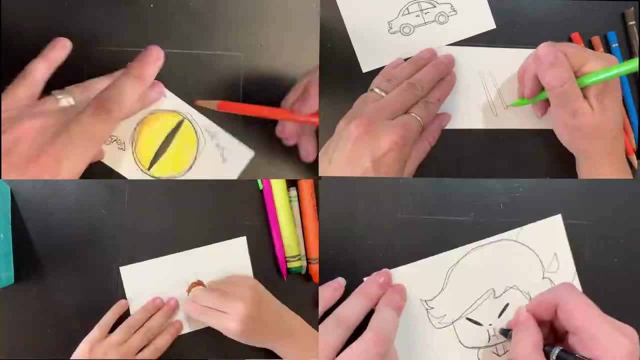 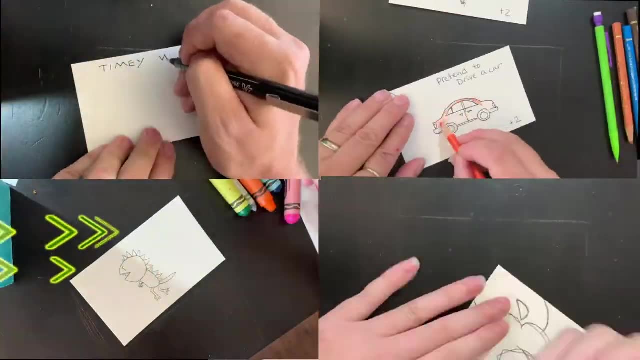 they're not working as well, or we can just keep adding and adding and adding. So maybe every time we play the game we'll make a couple more cards and then it'll be a fun surprise for everybody. as we're playing, We'll get to see new cards from new people. And there they are, Some of them. 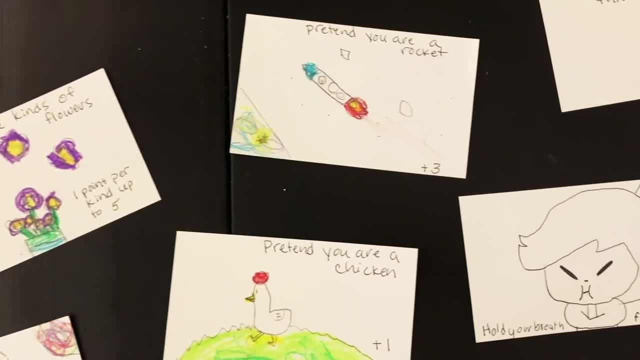 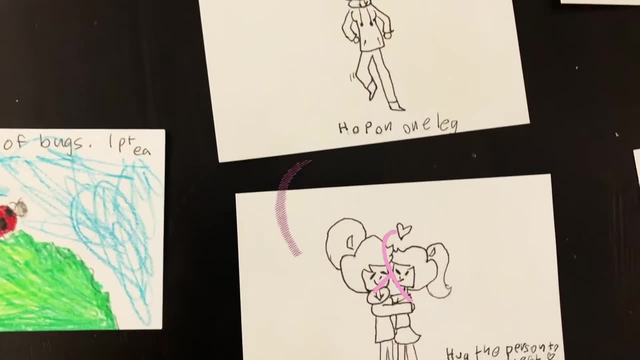 the finished ones. They turned out really nice. So act like a chicken, or pretend like you're blasting off In a rocket, or hold your breath, or hop on one leg, Or hug your neighbor. Hug your neighbor, That was a good one. 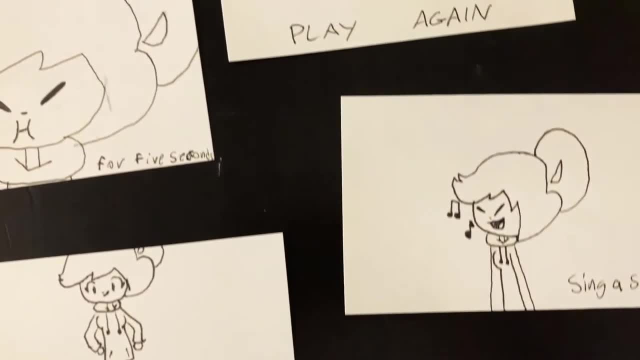 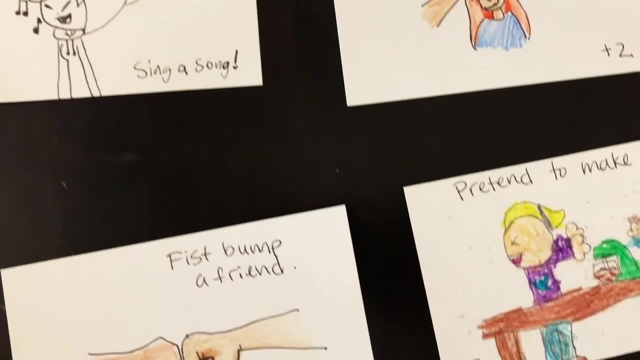 That was a really good one. Fist bump, Timey wimey, play again. There's the cracked phone screen, There's the pat, someone on the head and Sam's. pretend like you're baking, where one kid is throwing flour at the other kid. 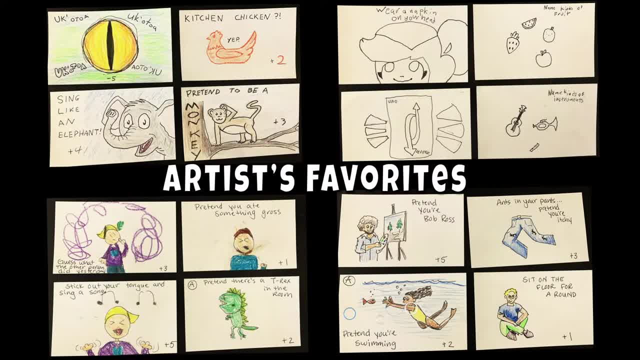 It's not the kid that's throwing it, It's the mixer. Oh, the mixer's throwing the flour. Where are? Where on earth would you have gotten that idea? Did that happen to us when we made our cookies? Yeah, Totally did, huh. 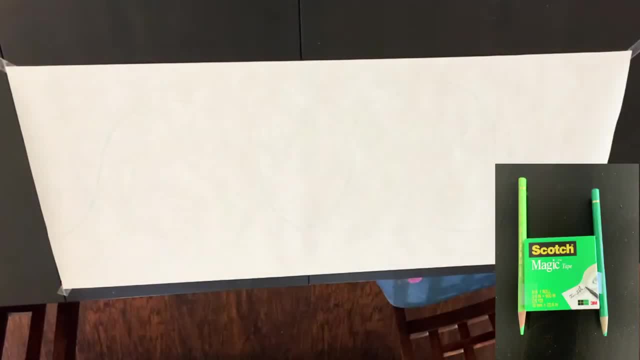 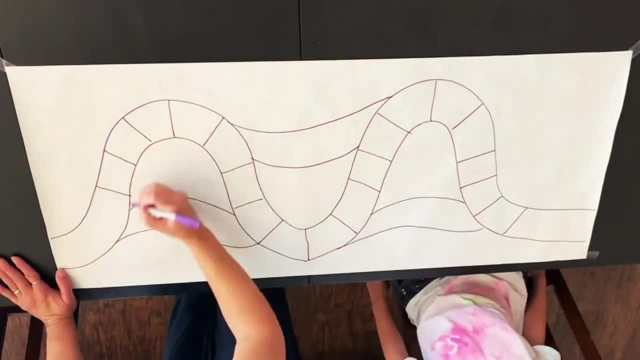 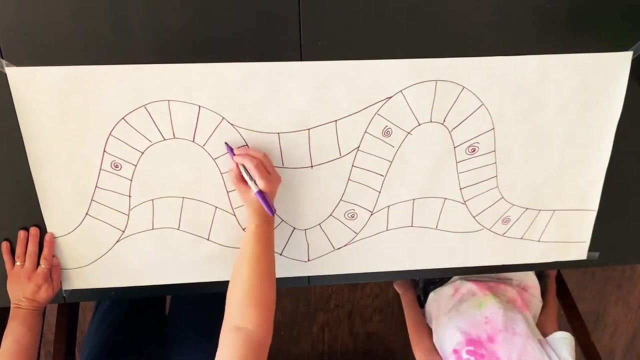 Okay, so this is when we made the game board. So at first there was that fancy tool that I used where I taped pencils to a box of tape to get the spacing kind of equal. Yeah, but it made it so that it was easy to get the spacing the same on the 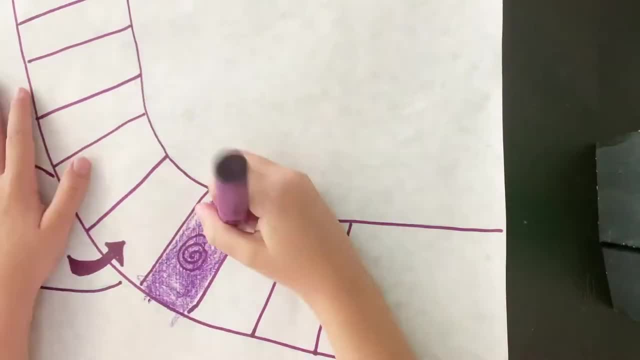 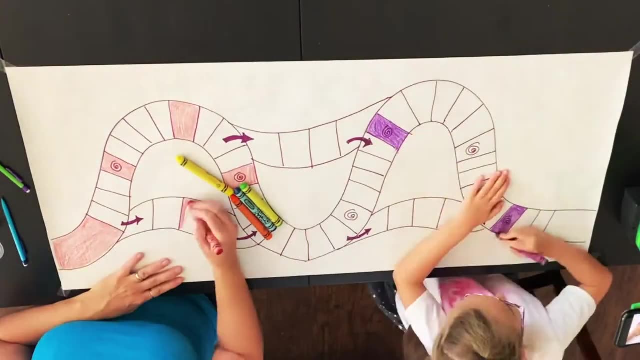 Totally unnecessary, but that's what we did, And then we kind of We were aiming for 42 spaces on our game board, So we just divided it up and then divided it up, and then divided it up so that we'd have that many spaces, And then we have the little swirly. 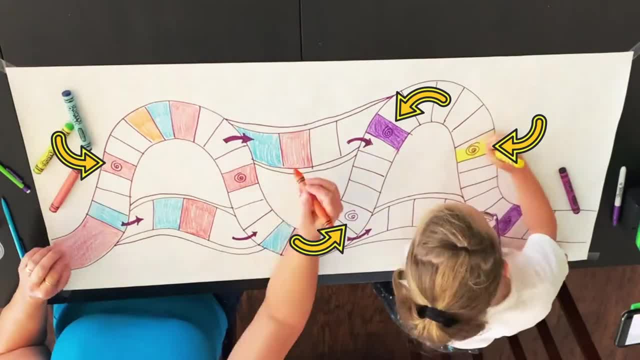 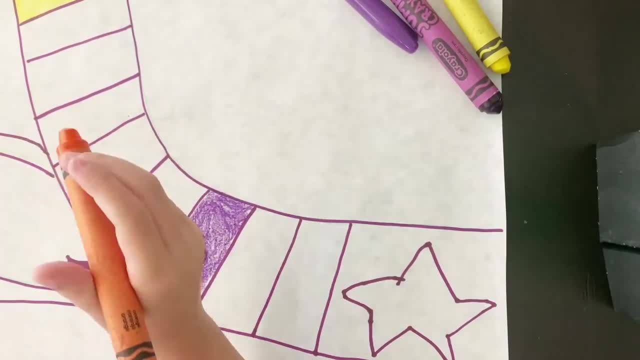 spots, which are teleporters, So if you hit one end you get to go to the other one, depending on the color. And then we also have the bridges with the arrows, which is fun to have shortcuts and sometimes you end up being sent backwards. I think it's fun, Makes it unpredictable, but it's. 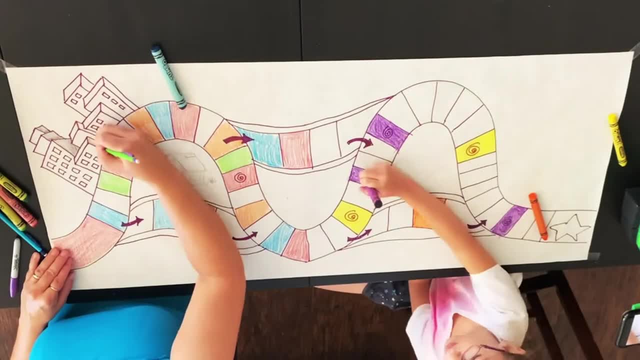 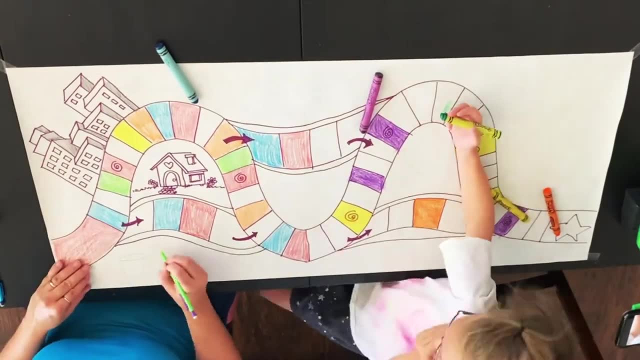 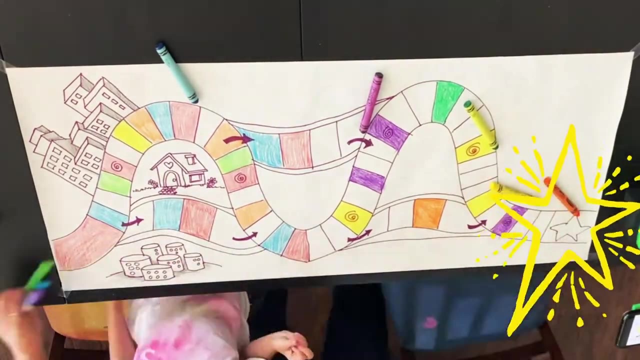 predictable. It means that even if you're ahead of the beginning of the game, you might not win at the end of the game. So Samantha was the all-star on the game board. coloring all the little spots. She drew the star for the end, for the dance party. We always have a dance party. 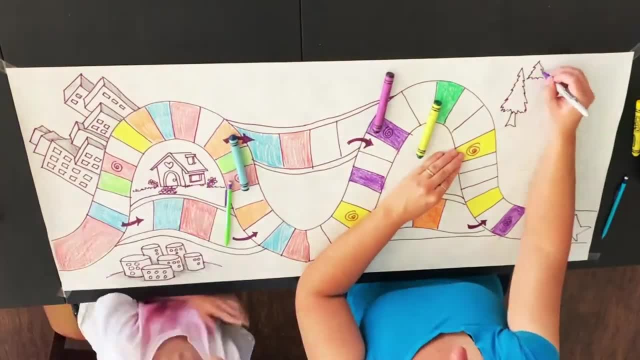 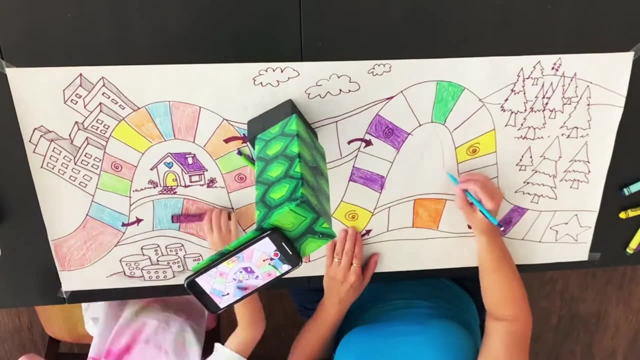 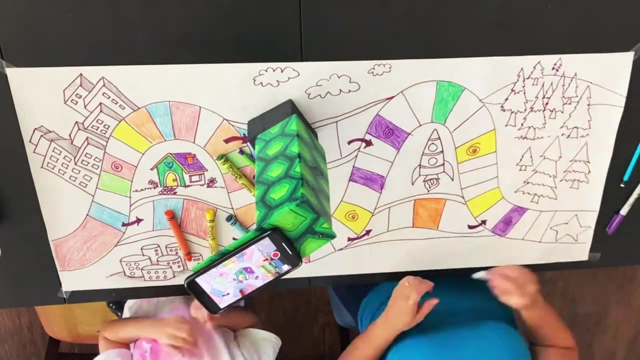 when everybody gets to the end. This is Steven Universe. Yeah, we ended up coloring a yellow star on a red background, so it's very Steven Universe. Yeah, What's your favorite part of the game board? Ty Um, I like the rocket ship. 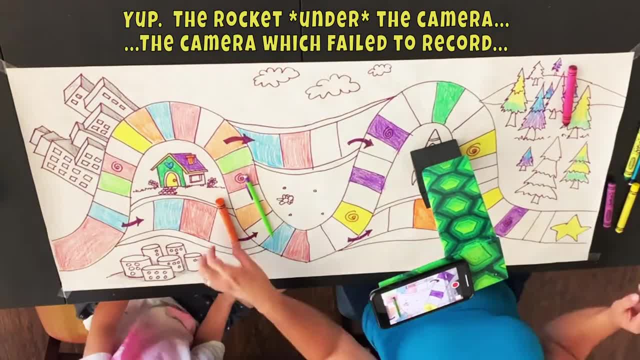 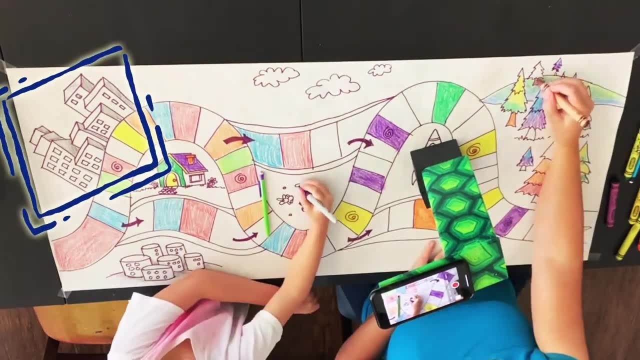 It turned out great. The rocket ship is a nice, nice little character, Yeah, and I, um Sam, was kind of telling me what to draw where. so we've got like the rectangular buildings and then we have the circle buildings and then we have triangle trees. That was what. 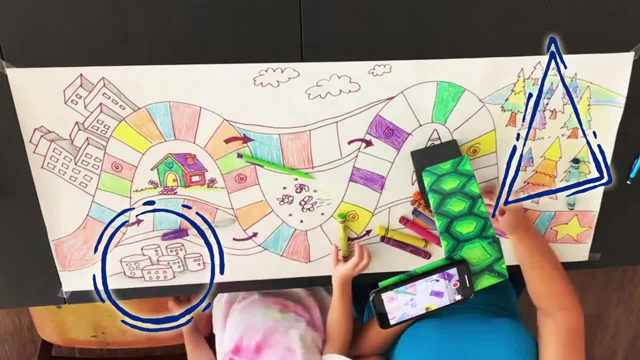 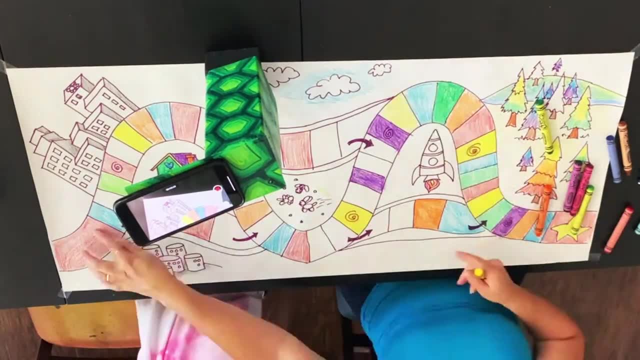 she wanted. And then um, Mythical trees. They're mythical. What did you draw on top of the roof? there I drew a little doggy sleeping on it And my kids are like: how did you get up there, you doggy? 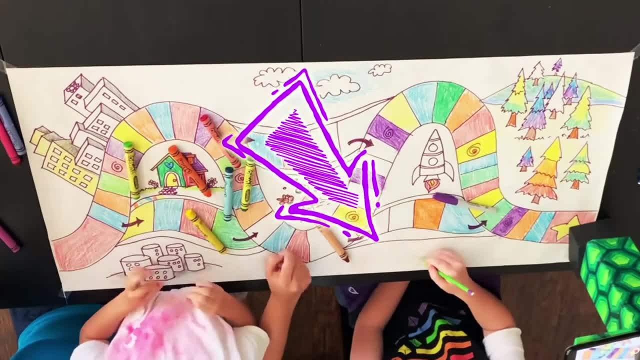 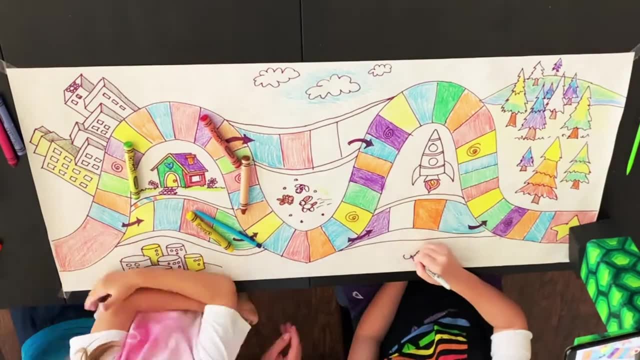 Yeah, Oh, here comes Ty. She's gonna draw the kitties on the bottom. Tell us about it, Ty. Purple is black. I got two of them like looking at each other and then one just laying on the ground playing. 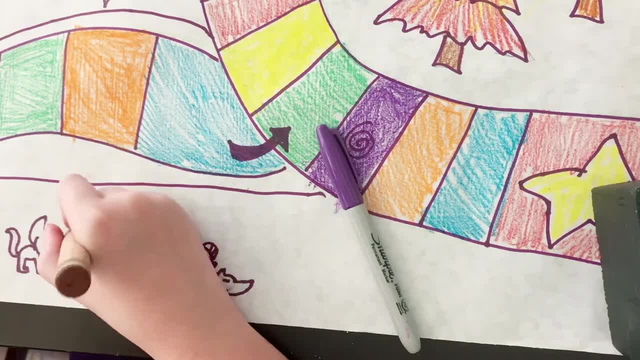 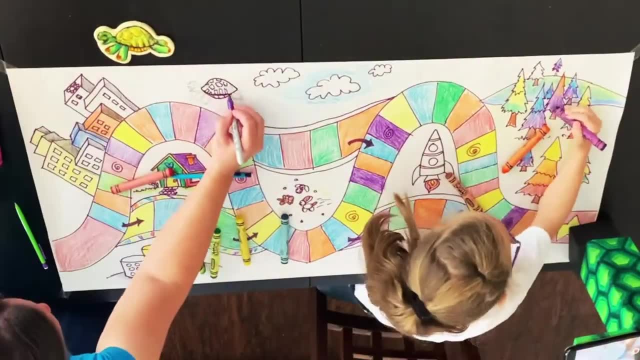 with a ball of yarn. That's adorable. And I used purple instead of black because We used purple outlines instead of black outlines. so, Mm-hmm, To make it more fun, And they're not. Purple kitty makes total sense. 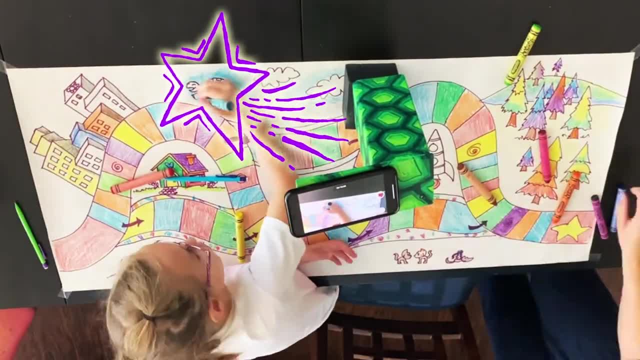 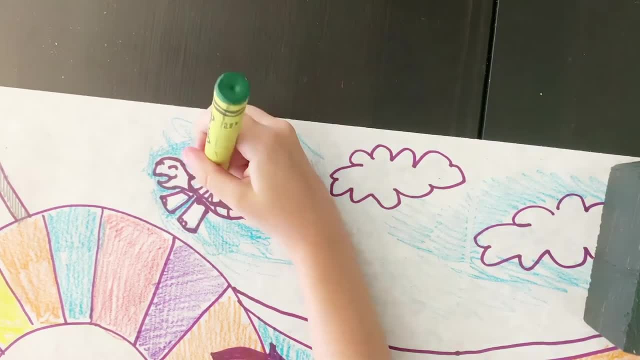 There's, there's Terry the tortoise flying around up there Over tortoise town, Of course, Of course. Now you're coloring the space, Yeah, Outer space. here we come, Adding the empty. Definitely the best part, For sure. And you did an ombre on the roof. 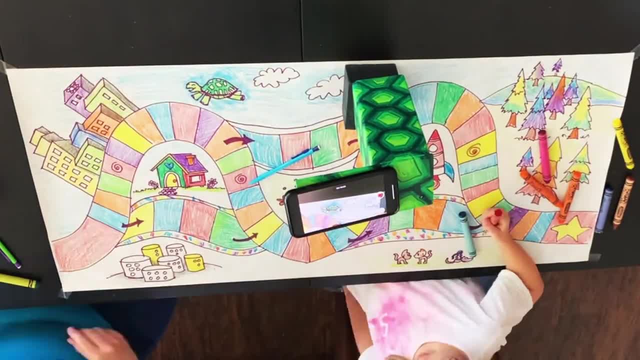 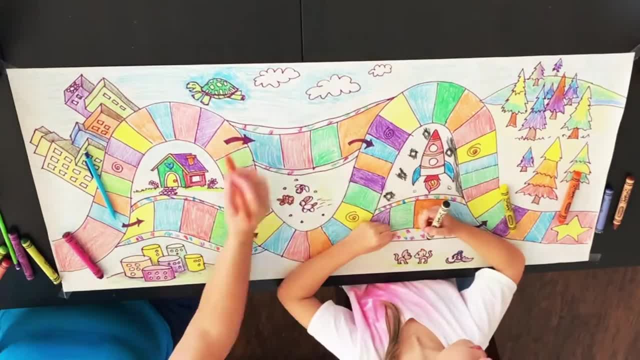 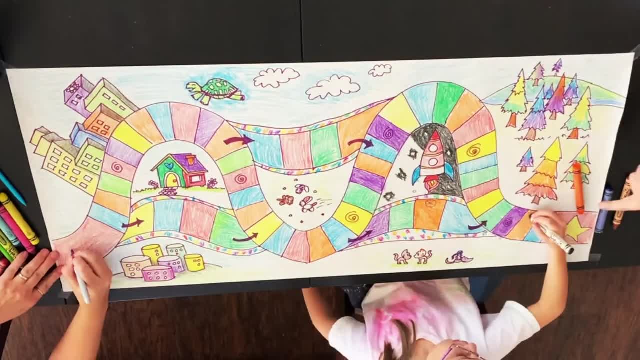 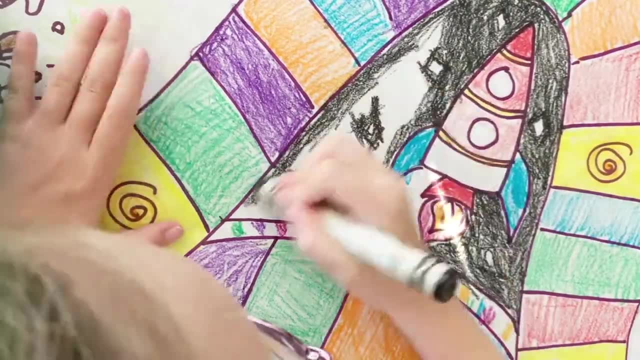 Yeah, Crayon For that whole thing. Yeah, That's awesome How I did it is. I pushed down on the first one and then, hey, it went a little lighter on the second one and then, and then the lightest, and then I went the lightest from. 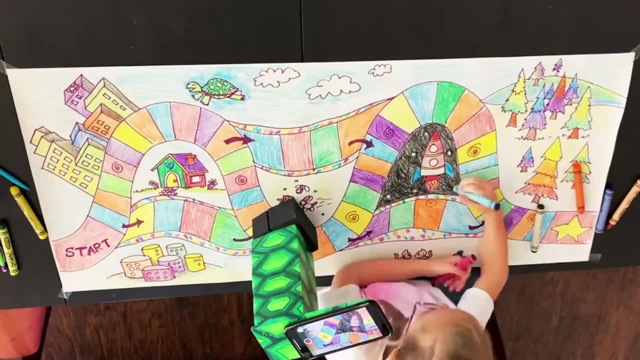 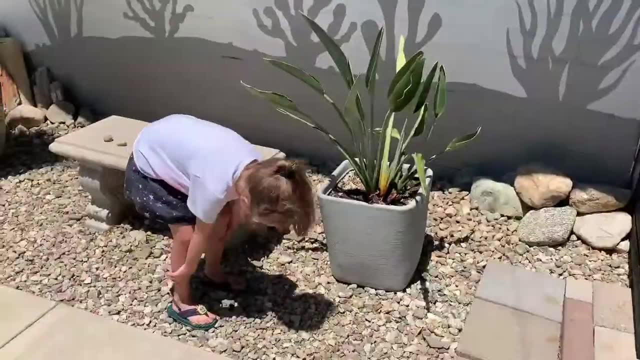 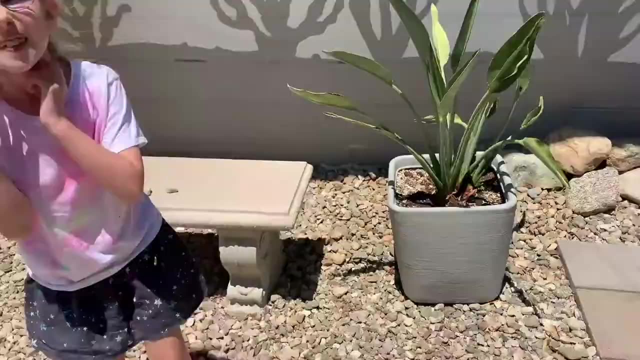 the, Yeah, From the, From the left, It's with this I'm picking out rocks. Yeah, I love that, I don't know. Yeah. so we gathered eight rocks. Four of them we used as game pieces and the other four we used to hold down the corners because our game board was a roll of paper. 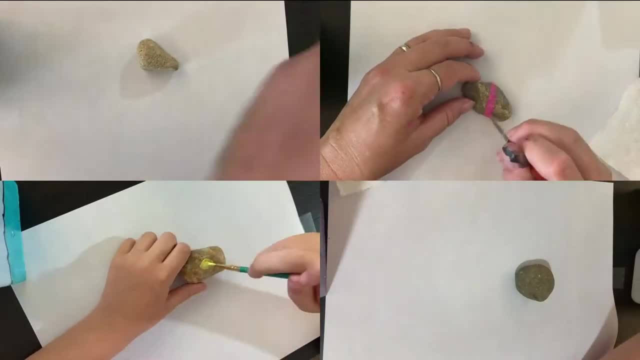 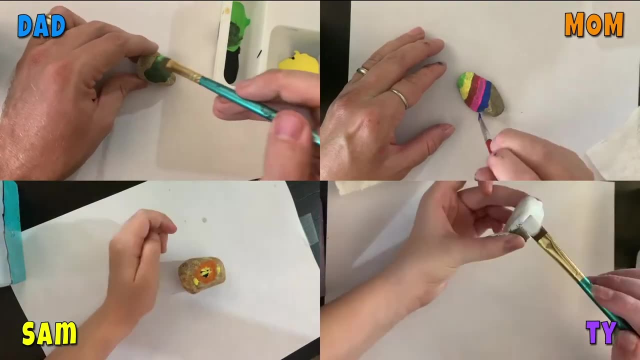 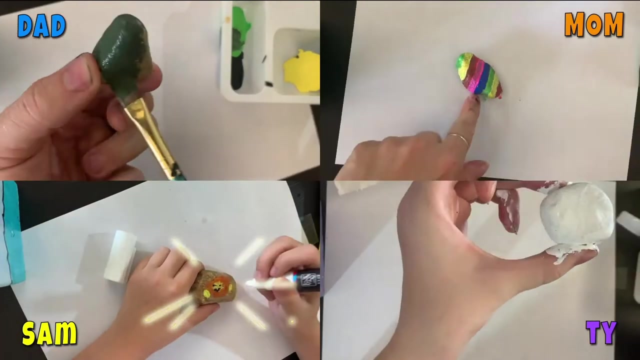 So we stuck them on the corner so it wouldn't unroll. But if we wanted to have more than four people playing, we could always do some of those for that. For my design, for my rock piece, I just painted a white base coat and then added some different colors, like a splotch thing: Purple and the blue-y color, The light blue. 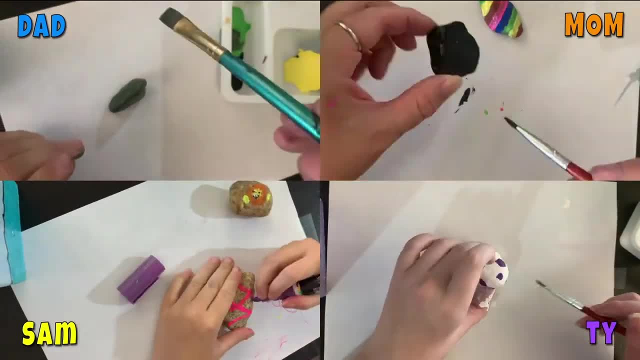 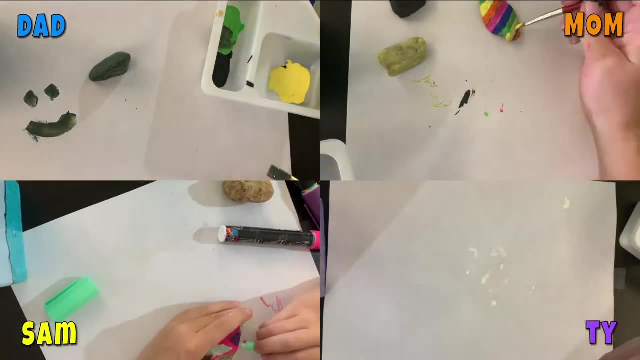 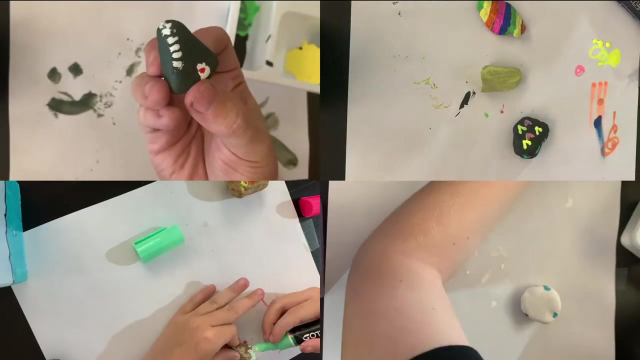 Nice, Okay, Sam, tell us about yours. I did a lion Because there's a lion in the Silly Street. one right, It's an homage. Mine's just a rainbow And mine's a dinosaur head, Which turns out to be fitting. 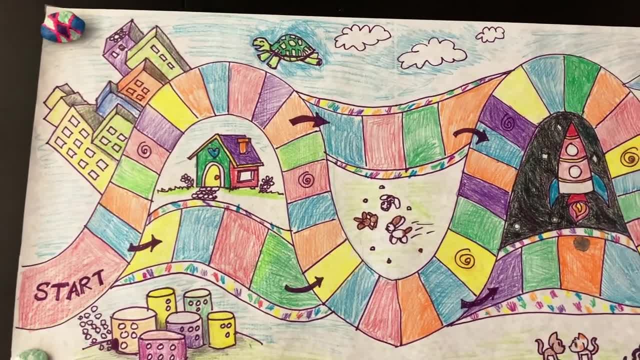 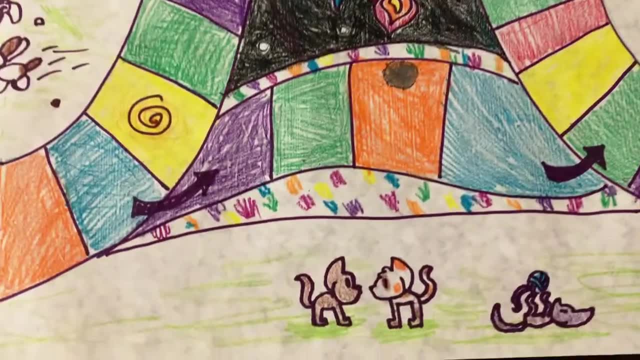 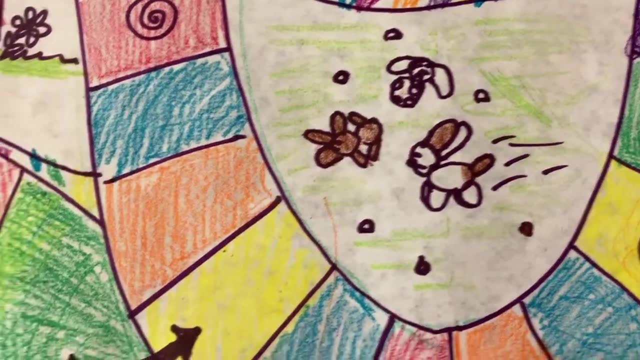 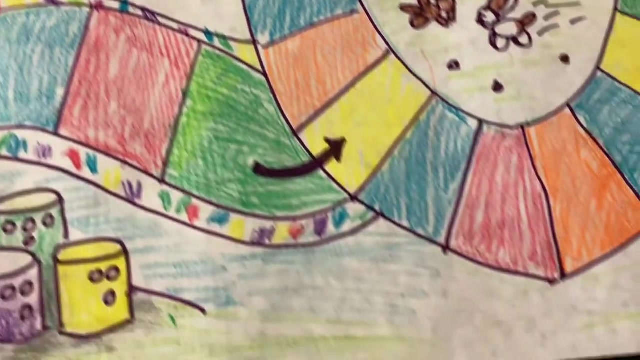 It does turn out to be fitting. There's the game board: nice and close, So pretty Space Over a rocket Happy town. Maybe that's Terry's house? Yeah, that's Terry's house, Terry's house. There's our game pieces. So there's Sam's lion. 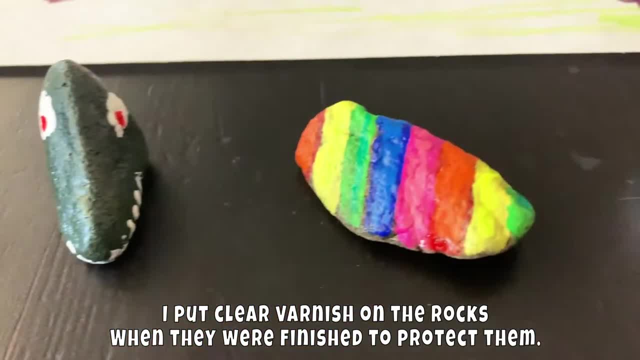 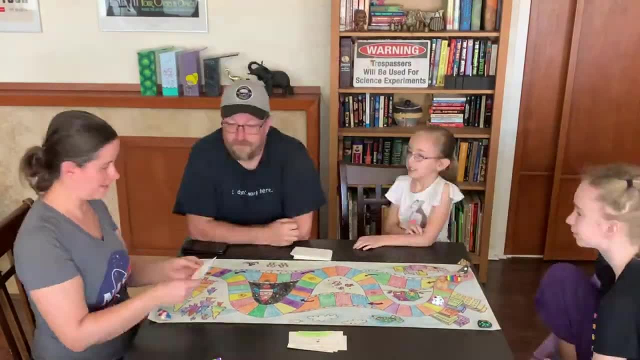 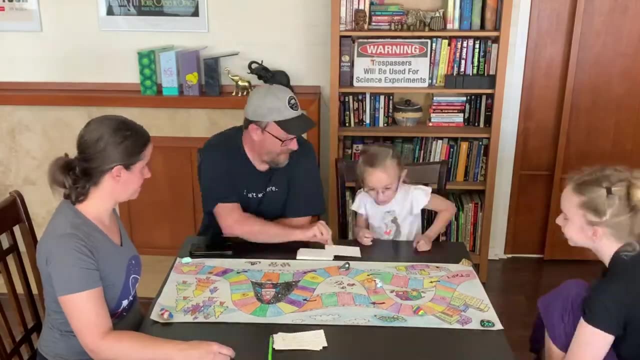 Daddy's dinosaur, I did a rainbow And Ty's splotches And we are playing. My favorite was when Sam was pretending to be Bob Ross and she said she was painting a happy little camphor tree Because we have a camphor in our yard to chase away the mosquitoes, and she's a fan. 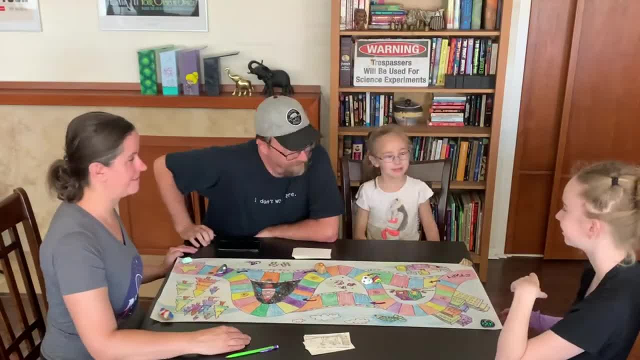 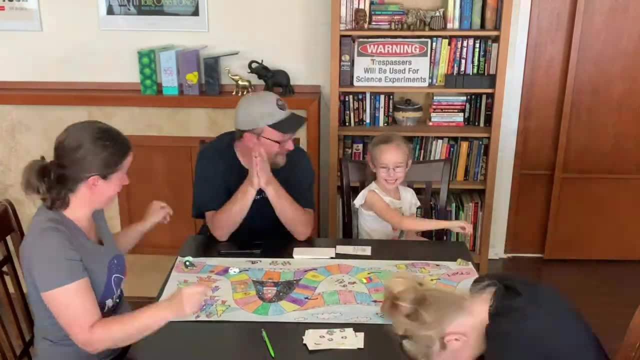 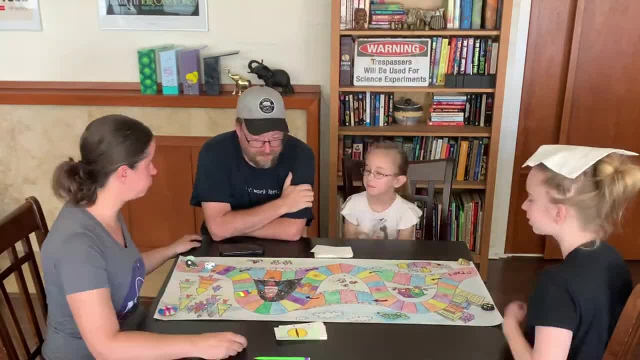 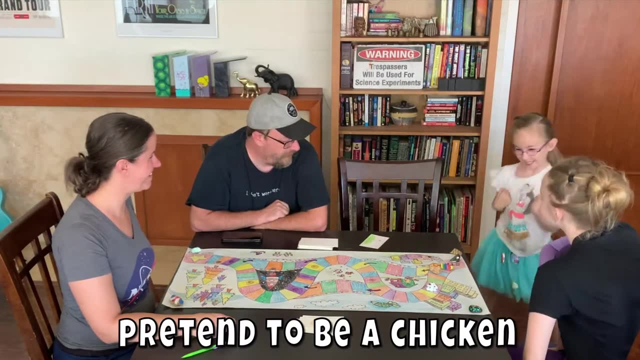 Bob Ross was awesome. No, no, no, Her chicken dance was pretty. Oh, her chicken dance was great, Pretty special, Pretty special. Yeah, She's a very enthusiastic chicken. All right, let's see it. Pretend you're a chicken. 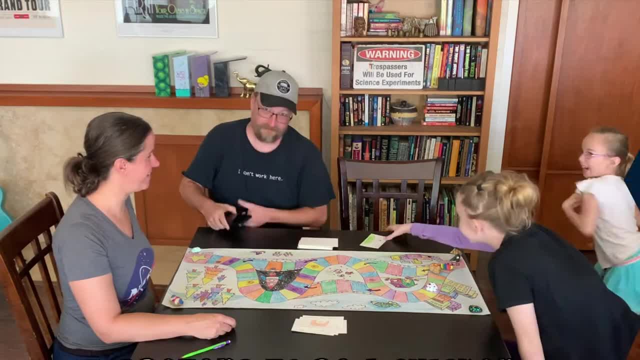 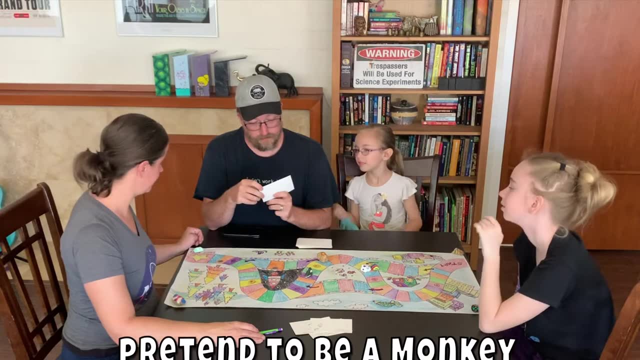 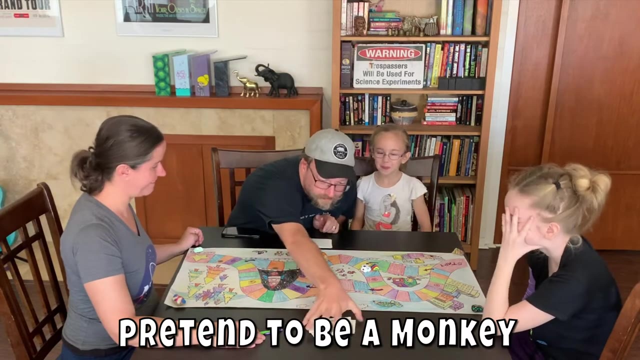 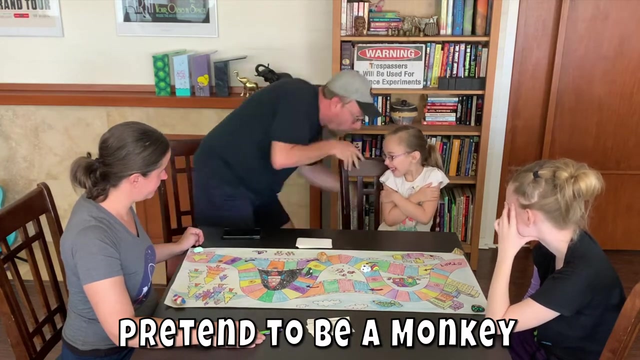 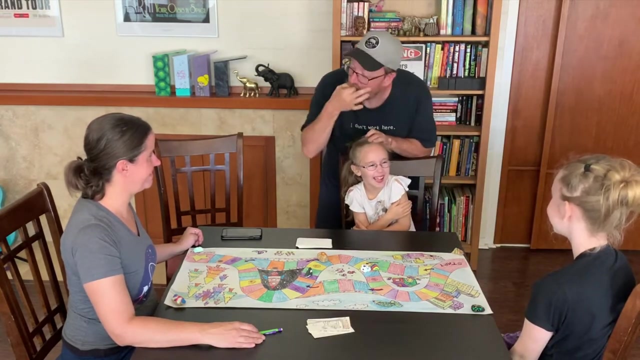 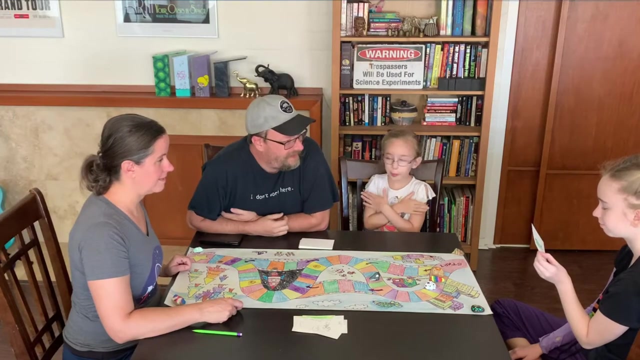 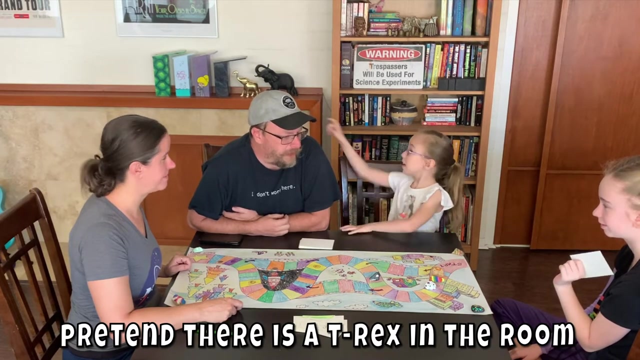 What does chicken say? There we go, There we go. I'm pulling all my cards. Pretend to be a monkey. That's a null play, right, Yeah, Okay, So where is it Right here? Haaah, there you go.